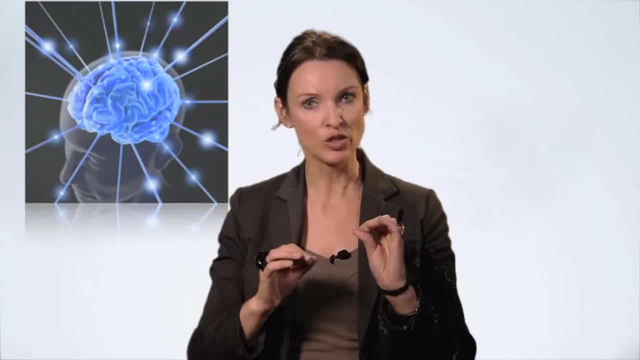 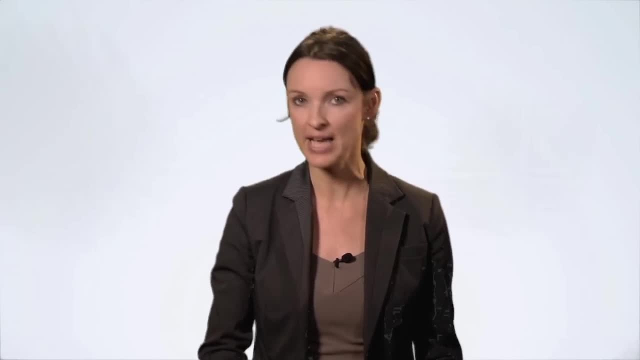 as having these different antennas, and your brain really wants to protect yourself and it takes that job very seriously. So as soon as the antennas perceive a kind of danger, a button is pushed. It's a button somewhere here in your head, in your brain, and it's. 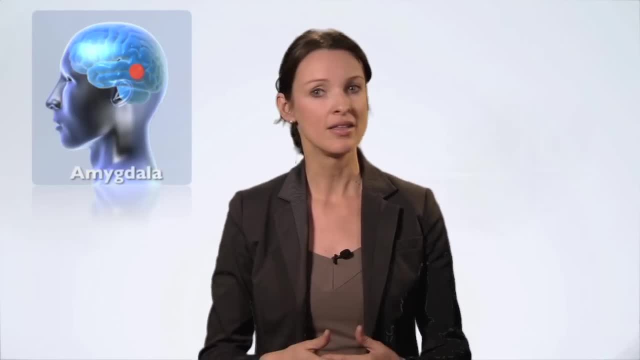 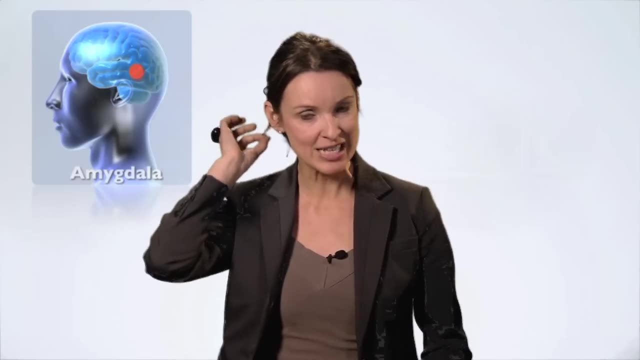 called the amygdala. It has the shape of an almond, the color of an almond. It is small as an almond, But it's a very important button. It's a very important button because as soon as the button is pushed, that's what we call. 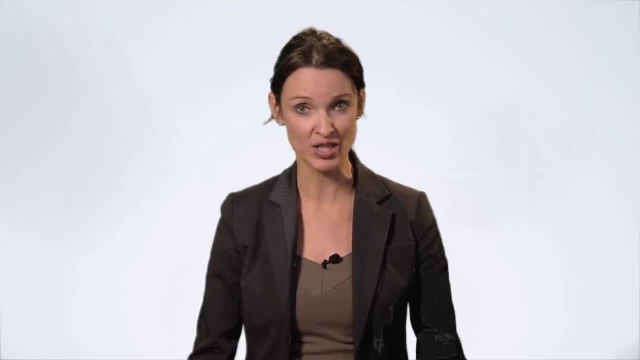 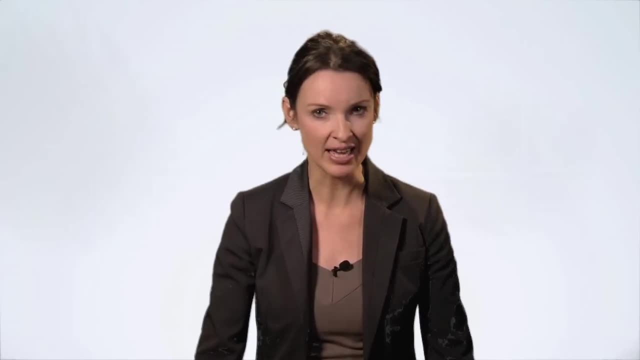 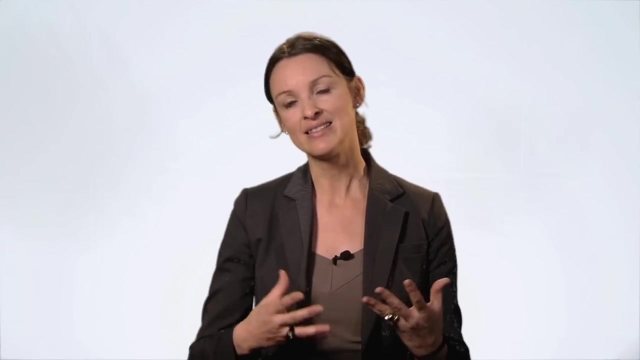 the fight-or-flight reaction. You have all these sensations in your body. typically the things that you experience when you are nervous, like a dry mouth, legs shaking, your heart really beating very fast. your respiration is going faster And this is something that 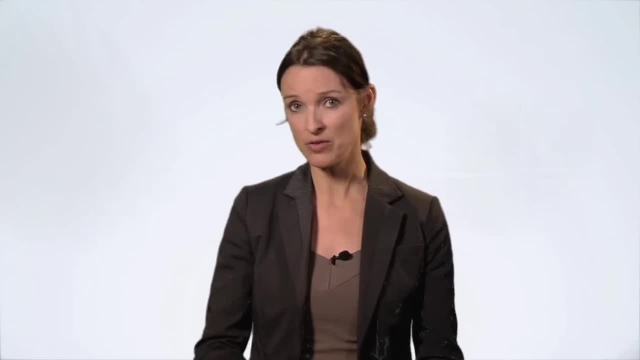 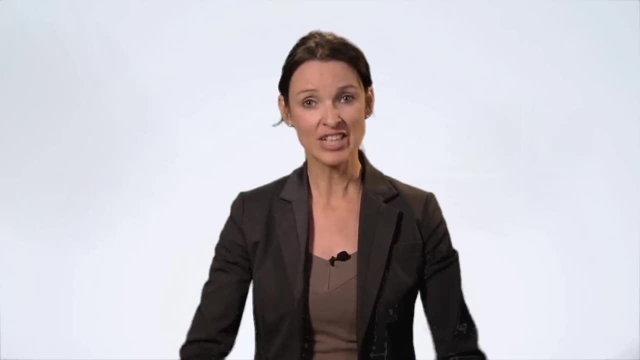 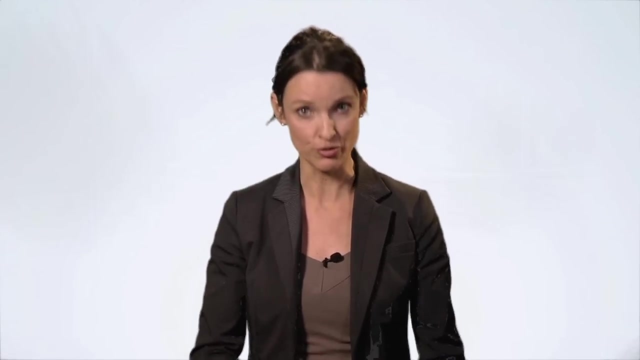 actually is there to protect yourself because, as it is a fight-or-flight reaction- imagine that there is this scar- It's really racing into you when you cross a road. The fact that you have this heartbeat, that is fast, it actually prepares you to react and to run. actually. 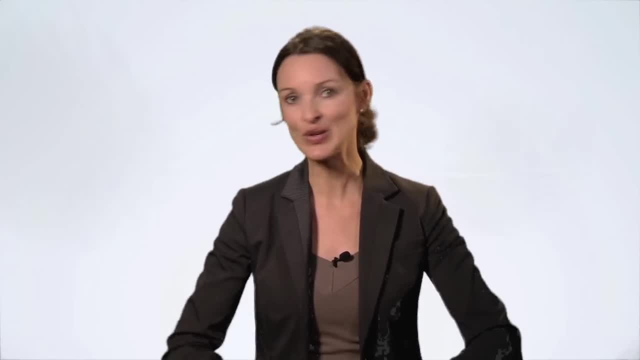 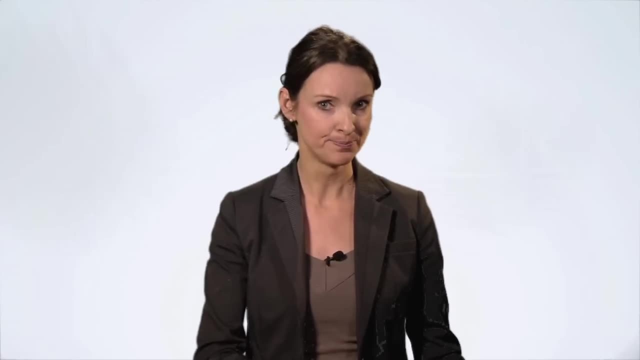 Now the thing is, when you stand in front of an audience you cannot run. So the antennas, they don't make a difference between a real danger and a danger in your head. So what happens is when you're in front of your audience you cannot run, You kind of freeze, but still. 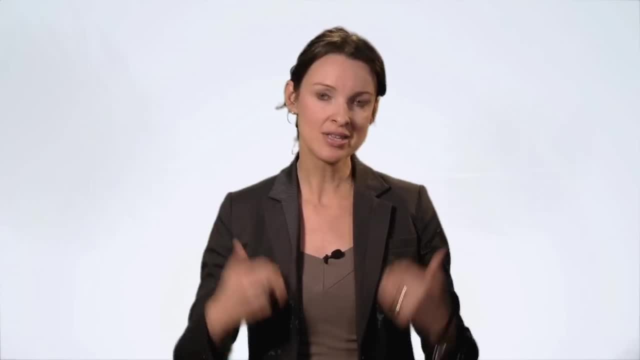 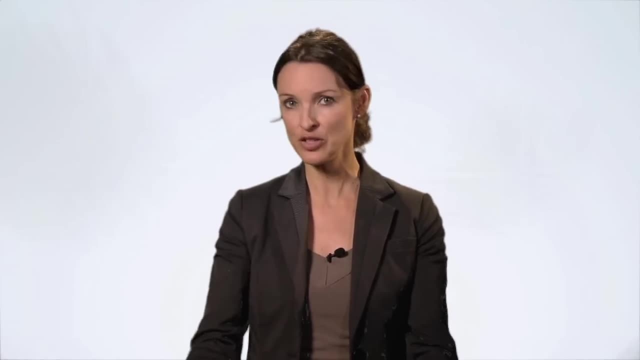 you have these sensations so you want to protect yourself. Now, this is on a subconscious level. What happens on a conscious level is that actually, when you stand in front of your audience, you want to protect yourself. so actually by doing this- Now this is overdoing. 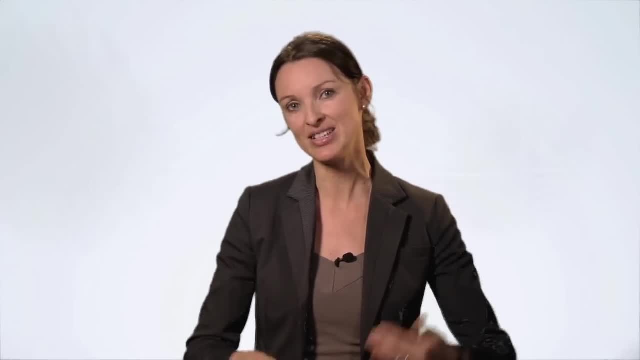 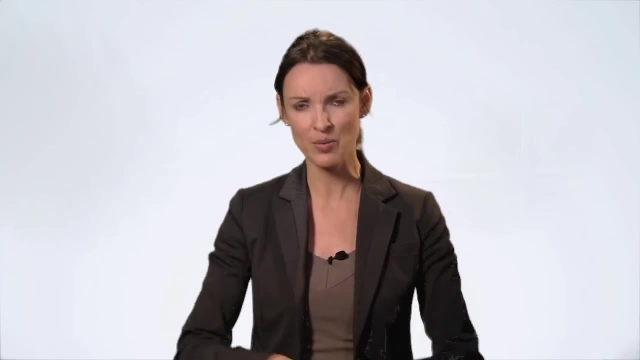 it, but to some extent that's what speakers actually do. in front of an audience, You stand like that. you really want to protect yourself, looking down or looking very quickly from one person to another. Now, what does an experienced speaker do? 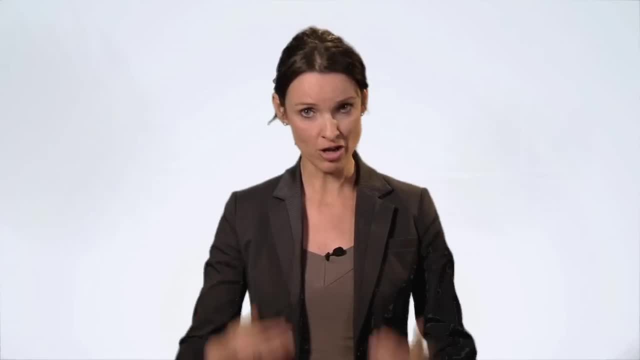 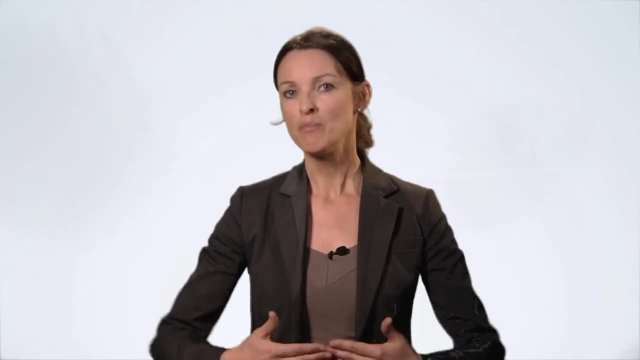 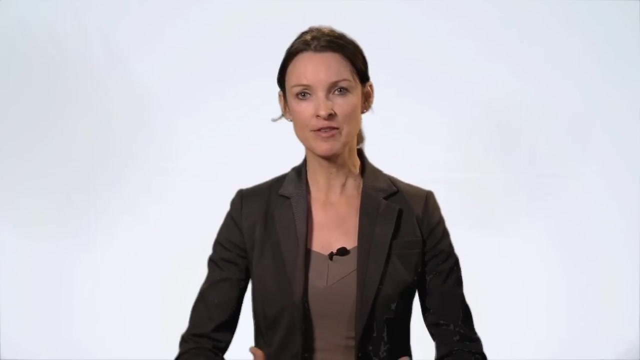 They do exactly the opposite. They, on a conscious level, they make themselves big in front of the audience. You could say that they fake it Making yourself big. what I mean with that is having that posture in front of your audience that gives you a kind of